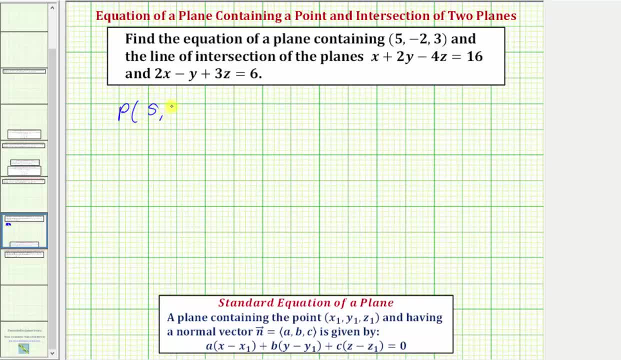 Let's call it. point p has coordinates five comma negative, two comma three. So we know, in the equation of our plane x sub one equals five, y sub one equals negative two, and z sub one equals positive three. So most of the work for this problem. 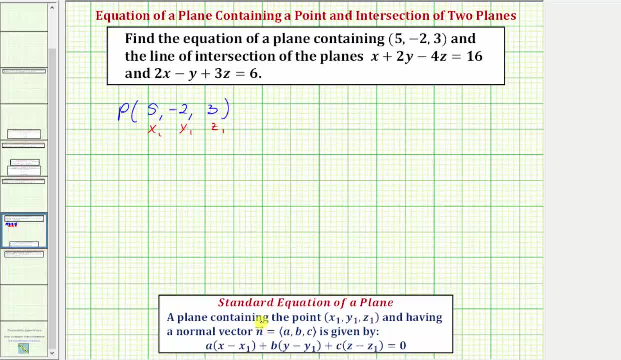 is determining a normal vector to the plane. To find this normal vector, we're going to find two points in the intersection of these two planes and then we'll use those two points and the given point to find two vectors in the plane. we're trying to find the equation of 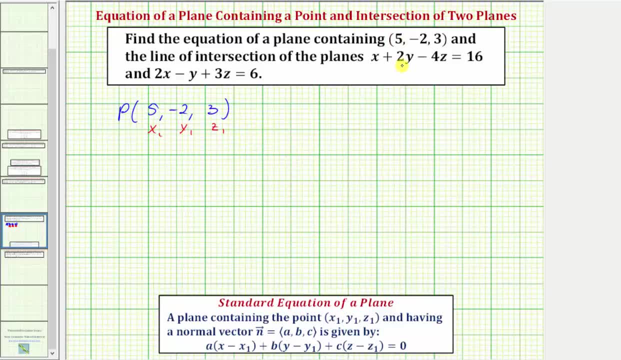 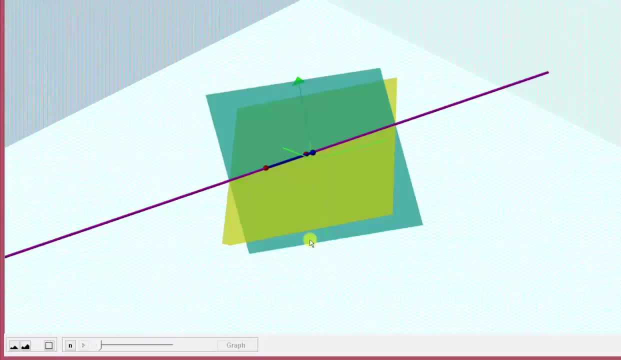 And then if we find the cross part of those two vectors, it'll give us a normal vector to the plane we want to find the equation of. To better understand this, let's look at this graphically. So here we see the graph of the given two planes. 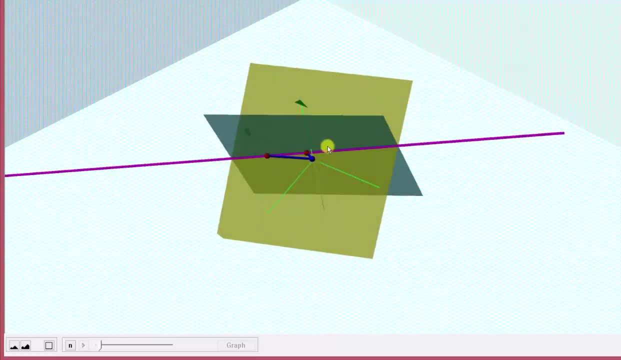 I've also graphed the line of intersection of the two planes, This blue point here is the point we're given, which is in the plane. we're trying to find the equation of. And again, what we're going to do is find two points. 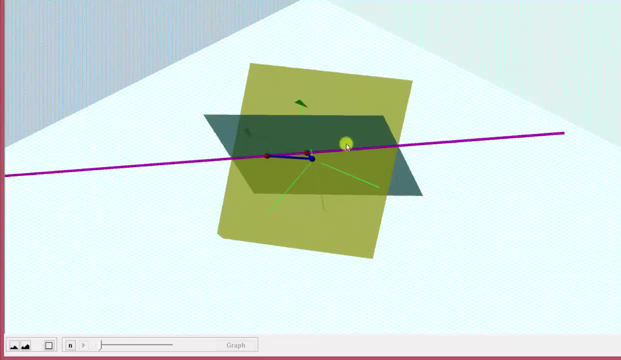 in the intersection of the two planes, or two points on this line of intersection. We'll use those two points to find two vectors in the plane we're trying to find the equation of which would be these two blue vectors. And if we find the cross part of these two vectors, 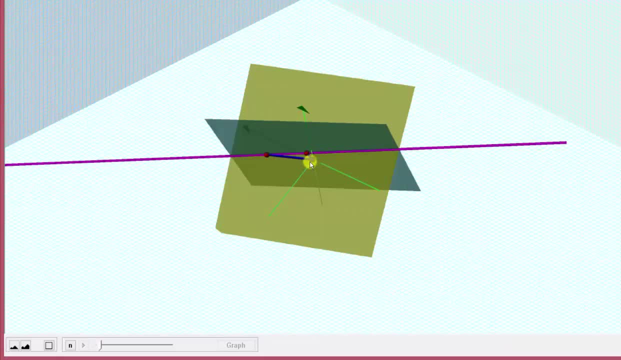 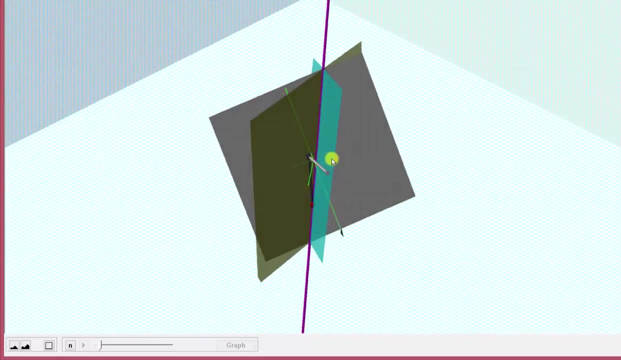 that cross product will give us a normal vector to the plane we're trying to find. the equation of The cross product of those two vectors would be this gray vector here And the plane we're trying to find the equation of is this gray plane here. 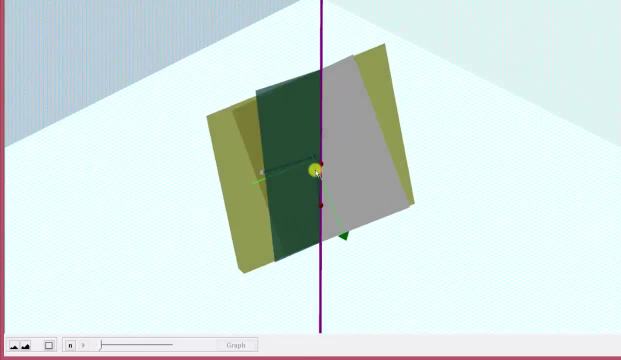 And notice how the gray vector is normal to the gray plane. So once we find the normal vector, we'll be able to find the equation of the plane containing the given point and also containing the line that is the intersection of the two given planes. 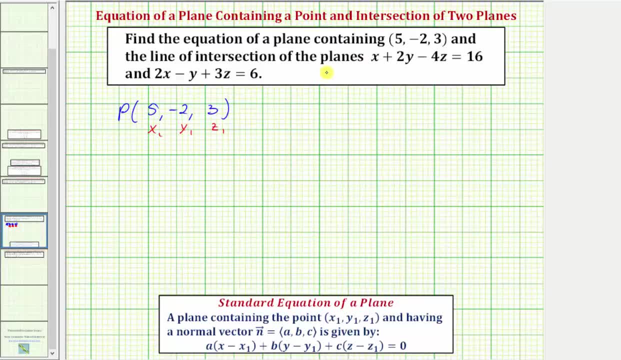 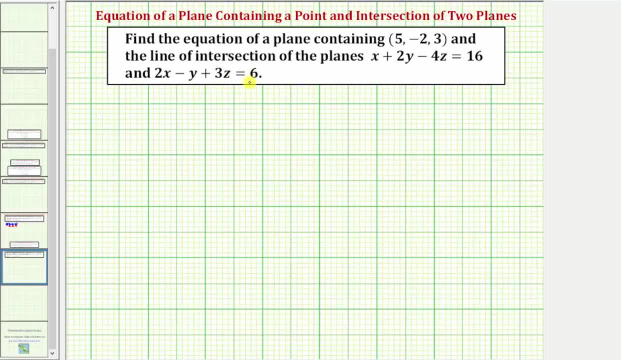 Now let's work on determining two points that would be in the intersection of these two planes, And we'll do this algebraically. For the first point, let's find the point in the intersection of these two planes when the x coordinate would be zero. 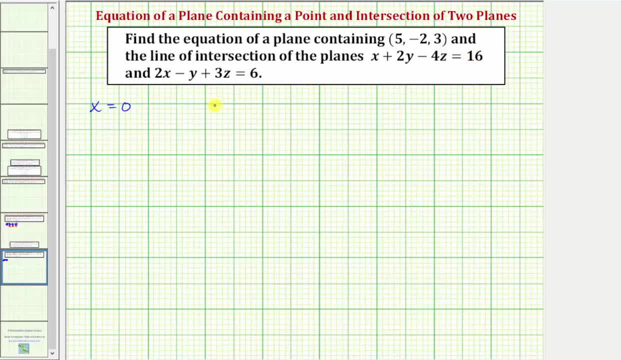 If we set x equal to zero, notice how this equation here would be two y minus four, z equals 16.. And this equation would be negative: y plus three, z equals six. Notice how, for this first point, I decided to let x be equal to zero. 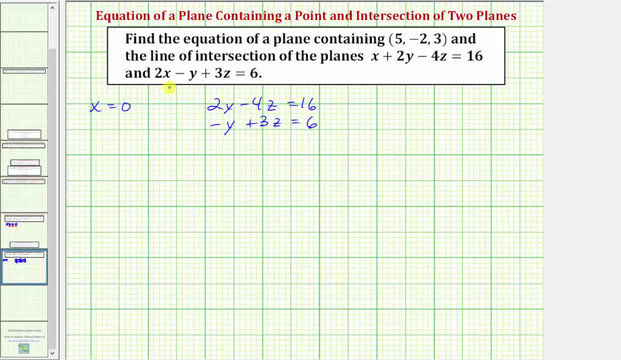 We can let any of the variables be equal to any constant and then solve for the two unknowns by solving the corresponding system of equations. Again for this first point, we're determining the point of intersection of these two planes when the x coordinate is zero. 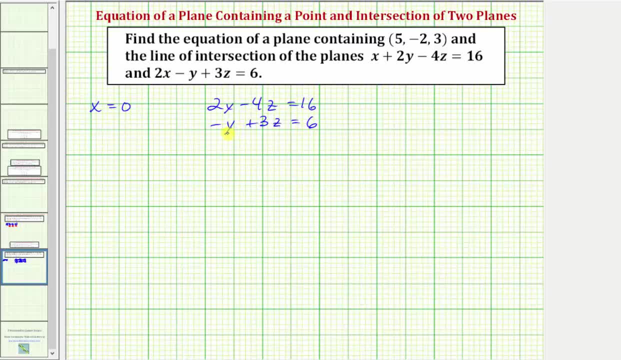 So we're going to do that. So solving this as a system, let's use elimination and multiply the second equation by two so we can eliminate the y terms. So if we multiplied the second equation by two and leave the first equation the same, 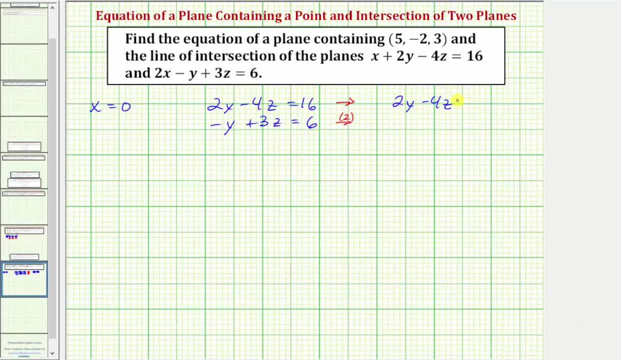 we would have two y minus four z equals 16.. And the second equation would be negative: two y plus six z equals 12.. Now if we add these two equations together, notice how the y terms are eliminated. this would be zero. adding the z terms, we get 2z equals. 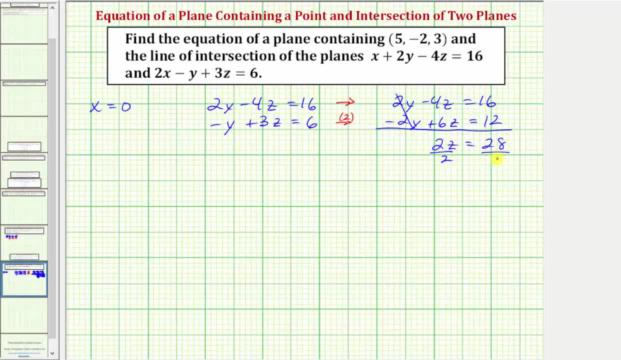 on the right side we have 28,. dividing both sides by two, notice how we have: z equals 14.. So when x is zero, we know z must be equal to 14, now we need to find the corresponding y coordinate by performing back substitution. 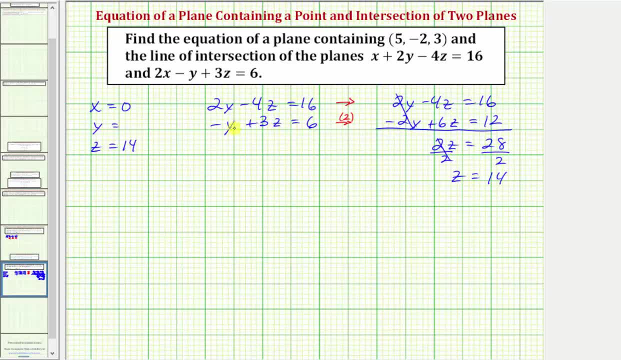 So substituting 14 for z in the second equation here we would have negative y plus three times 14 equals six. so we have negative y plus 42 equals six. subtracting 42 on both sides, we have negative y equals negative 36,. 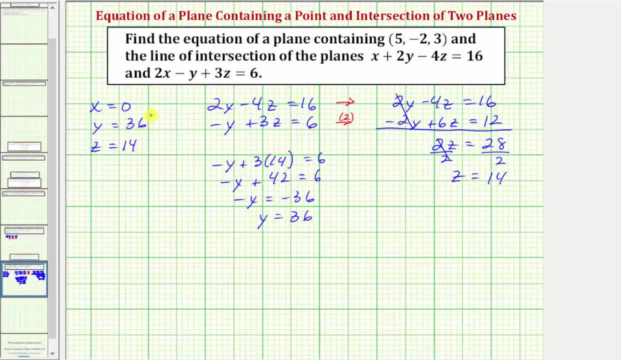 so y equals positive 36.. Which means one point on the intersection of the two planes is zero comma 36 comma 14.. And let's call this point B. Now let's find another point on the line of intersection of these two planes. let's find the point of intersection. 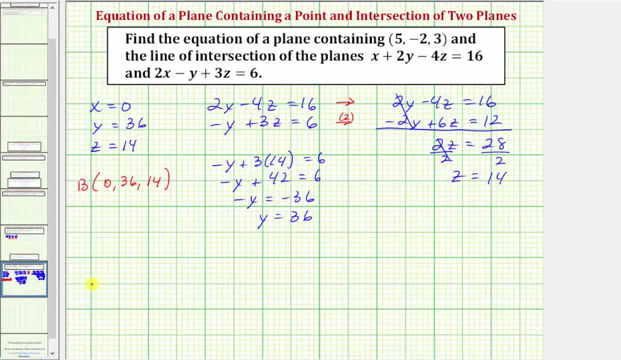 when, let's say, z equals zero. So we need to find the x coordinate and the y coordinate when z equals zero. Well, when z equals zero, this first equation would be: x plus two y equals 16.. and this equation here would be: two x minus y equals six. 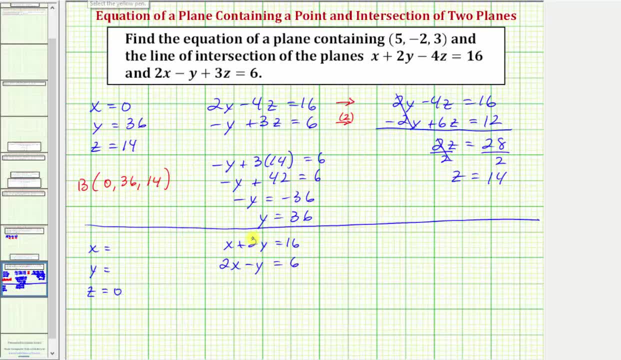 Again, let's go ahead and use elimination and eliminate the y terms. Let's multiply the second equation by two and leave the first equation the same. So we'd have x plus two y equals 16, and here we'll have four x minus two, y equals 12.. 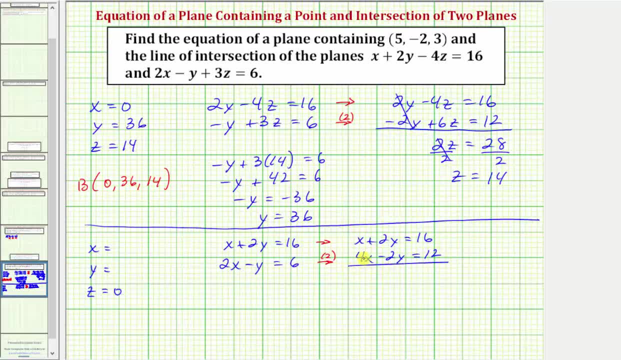 Adding the equations together, this would be one x plus four x, that's five x. The y terms are eliminated, so we have five x equals 28.. So we have x equals 28 fifths. So when z equals zero, x is 28 fifths. 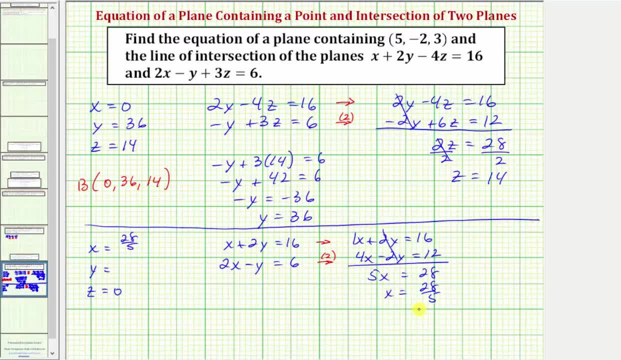 And I'll perform back substitution to find the y coordinate. Let's go ahead and use the first equation. So if x equals 28 fifths, the first equation would be zero. So that would be 28 fifths plus two. y equals 16.. 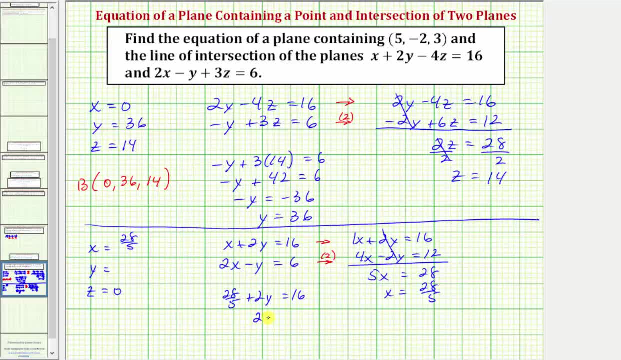 Subtracting 28 fifths on both sides would give us two y equals 52 fifths. Let's go ahead and multiply both sides by 1 1⁄2.. So here this simplifies to y on the right side, The two and the 52 simplify. 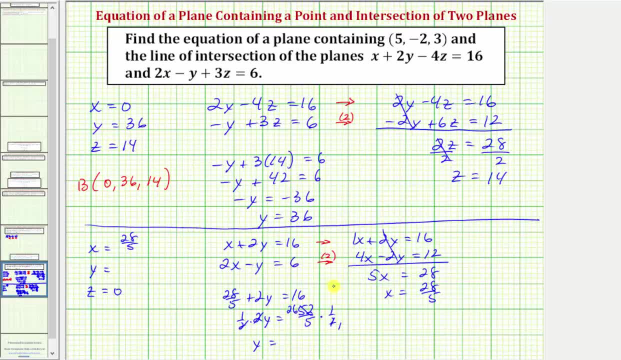 There's one two in two and 26 twos in 52. So we have y equals 26 fifths. So let's say point C, which would be a second point in the line of intersection of the two planes, has coordinates 28 fifths comma, 26 fifths comma zero. 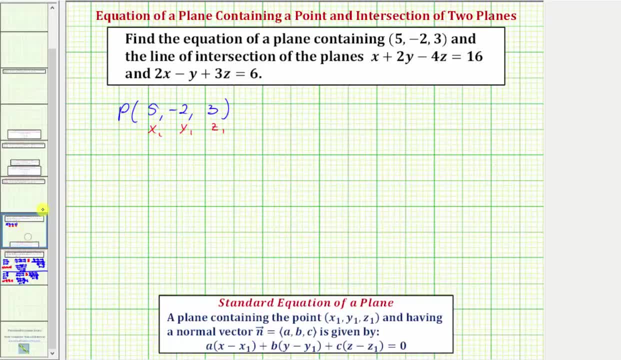 So now, using these two points that we just found, and the given point we know is on the plane, we'll form two vectors, then find their cross product, which will give us a normal vector, which will give us a normal vector, which will give us a normal vector. 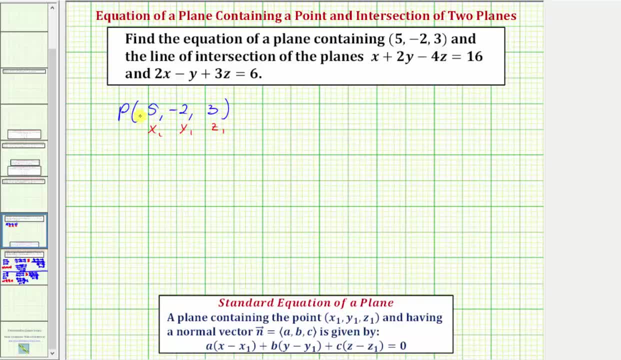 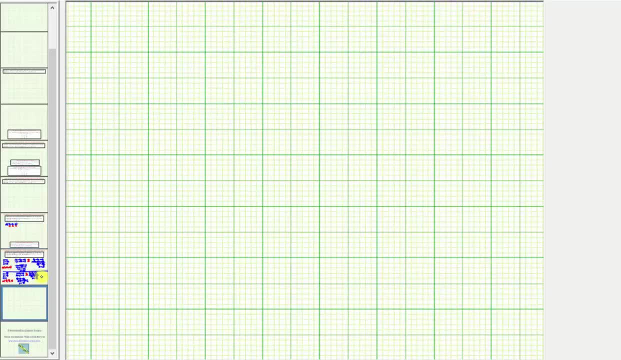 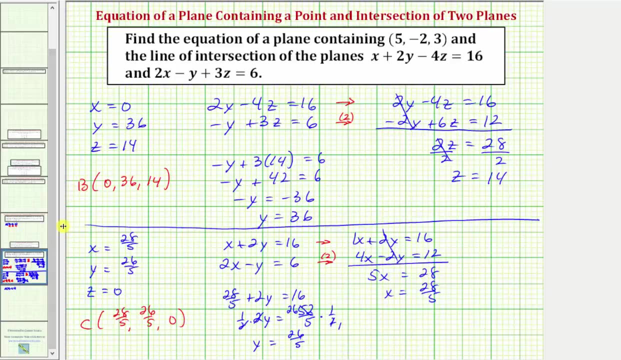 to the plane. we're trying to find the equation of: So for the given point, instead of calling it point P, let's go ahead and call it point A. So we know, point A has coordinates five comma negative, two comma three. Point B has coordinates zero comma, 36 comma 14.. 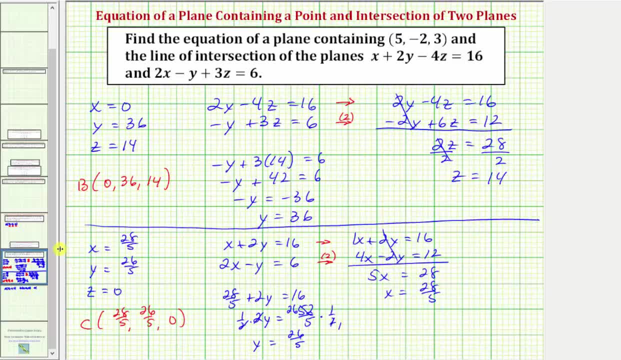 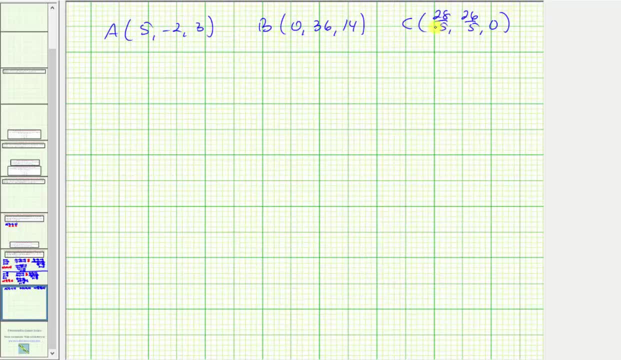 And point C has coordinates 28, fifths comma, 26, fifths comma, zero. Now I do want to point out that point B and C can be any two points on the line of intersection of the two planes. We found this point by setting x equal to zero. 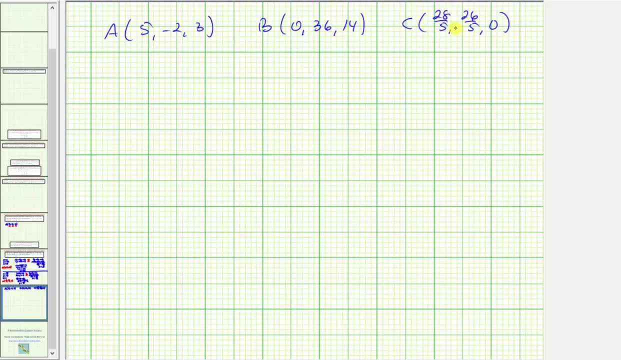 and solving for y and z. And we found this point by setting z equal to zero and finding x and y. But remember, we could let x, y or z be equal to any constant and solve the resulting system of equations in order to find any two points. 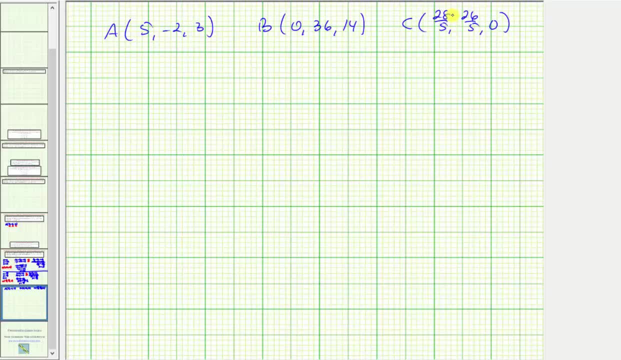 on the line of intersection. Now we'll form two vectors that are in the plane. we're trying to find the equation of. We have vector AB and also vector AC. So vector AB in component form would be zero minus five comma 36 minus negative two. 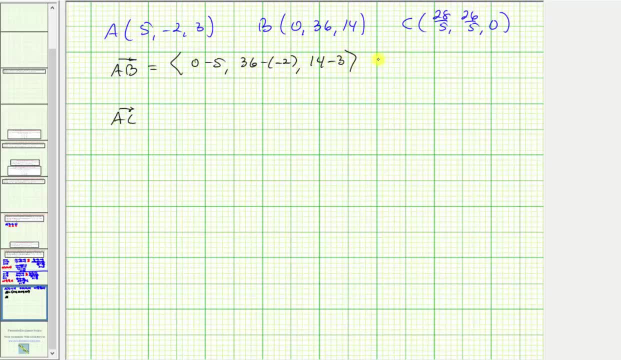 comma 14 minus three. So in component form vector AB would have components negative five comma 38 comma 11.. Let's let vector AB be vector V sub one, So vector V sub one is one vector in the plane. we're trying to find the equation of. 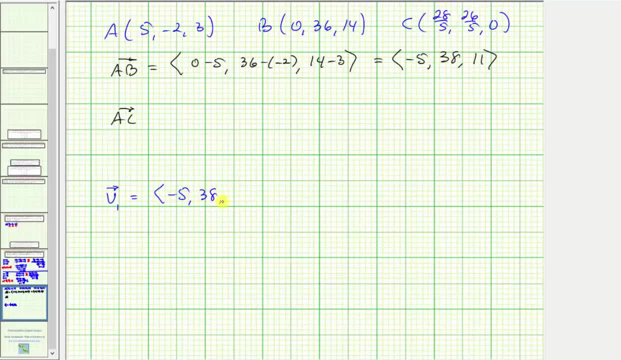 which again has components negative: five comma 38 comma 11.. And now let's find the component form of vector AC. Vector AC would have components 28 fifths minus five comma 26 fifths minus negative, two comma zero minus three. So simplifying: 28 fifths minus five. 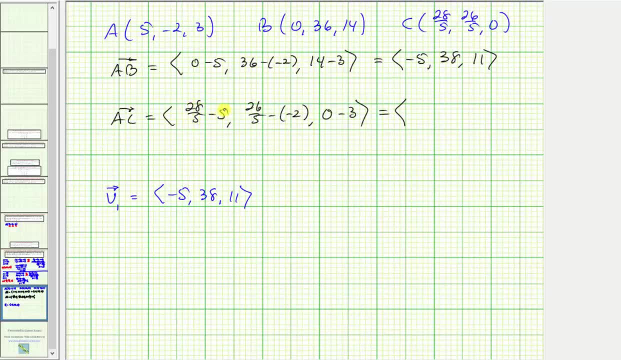 is the same as 28 fifths minus 25 fifths, which would be equal to three fifths. 26 fifths plus two is the same as 26 fifths plus 10 fifths, which would be 36 fifths, And zero minus three is negative three. 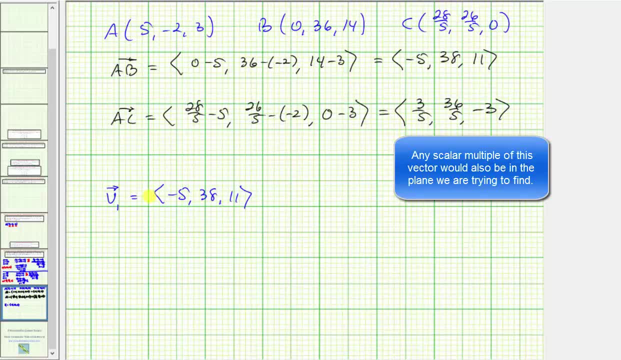 To clear the fractions, though, let's set the second vector in the plane. we're trying to find the equation of be vector V sub two, which equals five times vector AC, Because, remember, we do have to find the cross product of these two vectors. So vector V sub two. 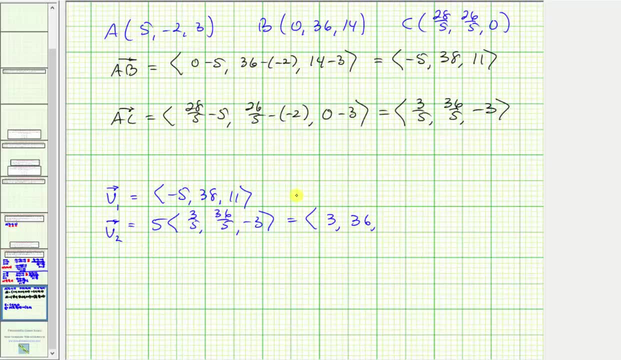 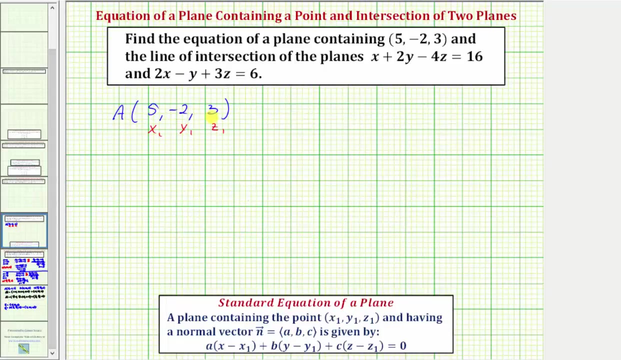 would have components three comma, 36 comma, negative 15.. And again, now we'll find the cross product of these two vectors, which will give us a normal vector to the plane. we're trying to find the equation of. So, going back to our very first slide, 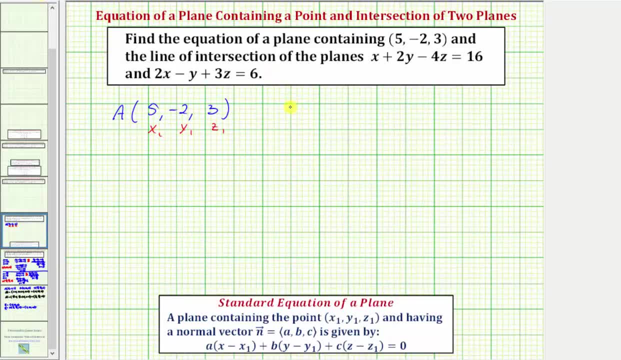 we know, point A is a point in the plane And now we're going to find a normal vector to the plane by determining the cross product of vector V sub one and vector V sub two, And let's do this on the next slide. We'll determine the cross product. 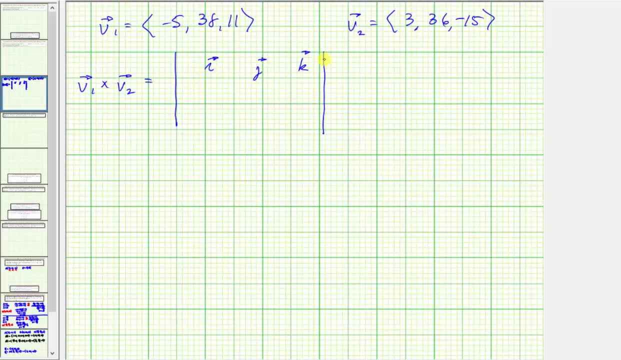 by setting up this three by three determinant, where the first row of the unit vector is I, J and K, The second row will be the components of vector V, sub one. The third row will be the components of vector V, sub two. And now we'll evaluate this using expansion by minors. 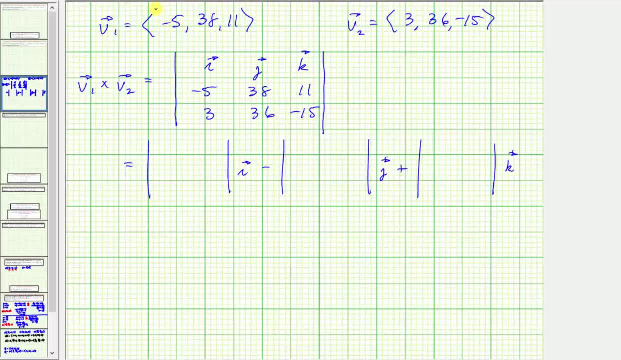 For the elements of this first, two by two determinant, we eliminate the row and column of the I vector, which would be row one, column one, So we have 38,, 11,, 36,, negative 15.. For the second determinant, 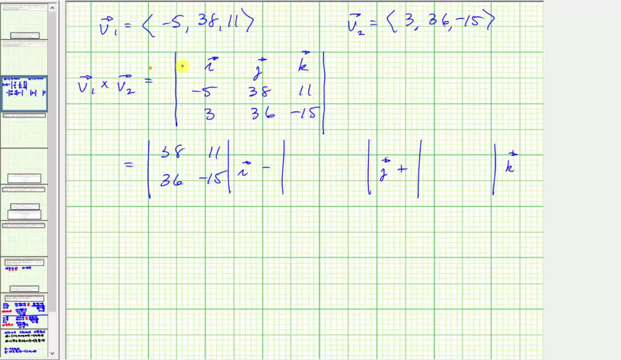 we eliminate the row and column of the J vector. So, row one, column two, Remember this is minus here. So we have negative five, 11, three, negative 15.. And for this last two by two, determinant, we eliminate the row and column of the K vector. 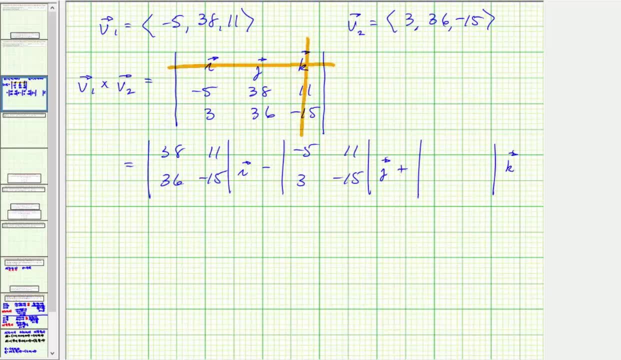 So we eliminate row one, column three. So we have negative five, 38,, three, 36.. And now, for each two by two, determinant, we're going to find this product minus this product In component form. the S component is negative 966.. 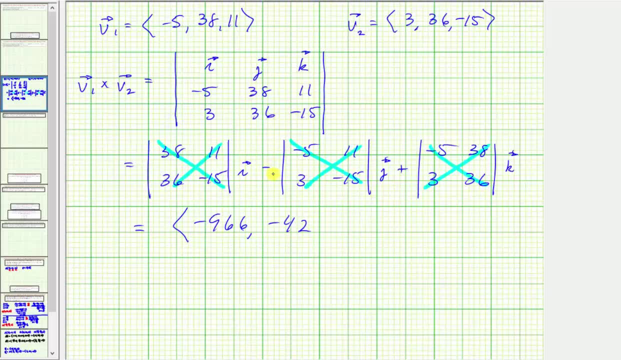 The Y component is negative 42. Be careful of the minus sign here. And the Z component of negative 294.. So this vector is normal to the plane. we're trying to find the equation of, But so is any scalar multiple. So let's set our normal vector N. 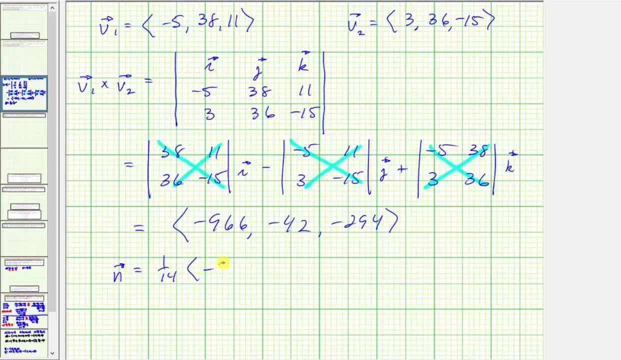 equal to 1, 14th times. this vector 14 happens to be the greatest common factor of these three numbers. So this would give us an X component of negative 69, a Y component of negative three and a Z component of negative 21.. 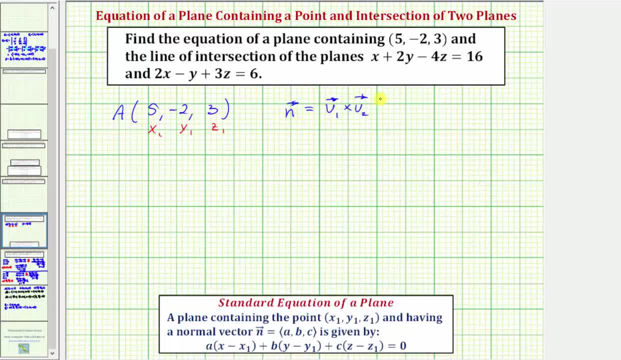 So, finally, going back to our first slide, we now know a normal vector to the given plane. So for the equation of our plane that contains this point, as well as the line of intersection of these two planes, we now know a equals negative, 69,. 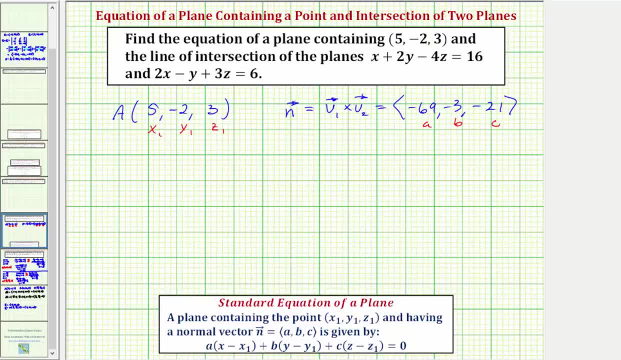 b equals negative three and c equals negative 21.. So the equation of the plane is negative 69 times the quantity X minus five, minus three times the quantity Y plus two, because we'd have minus negative two, and then minus 21 times the quantity Z minus three. 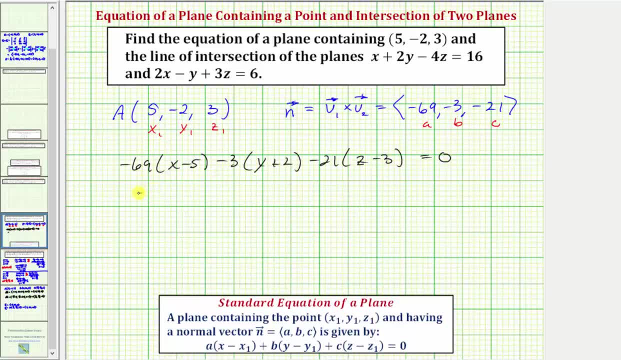 equals zero. Let's go ahead and distribute: We have negative 69 X plus 345 minus three Y minus six minus 21 Z plus 63 equals zero. Combining like terms, we'd have negative 69 X minus three Y minus 21 Z. 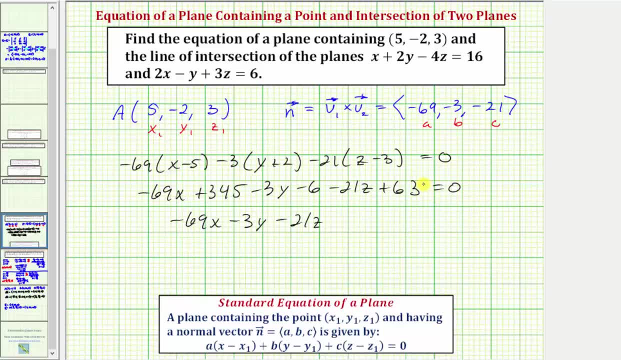 Combine the constants, we have 345 minus six plus 63, which equals 402.. Let's go ahead and multiply through by negative one and move the constant to the right side. That would give us 69 X plus three, Y plus 21 Z equals 402.. 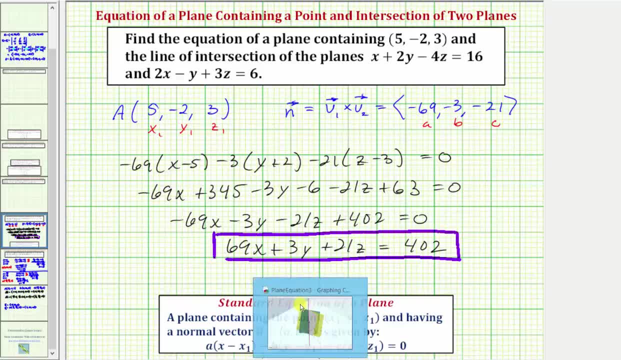 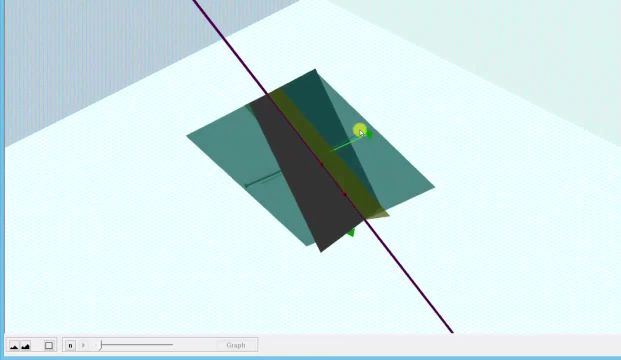 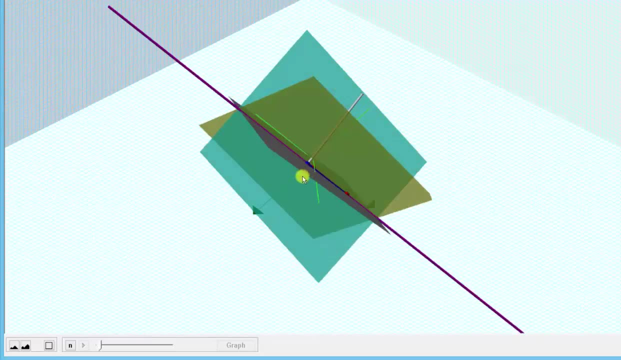 So, going back to our graph, one last time, the graph of this equation would be this gray plane that contains the given point, which is this blue point right here, and also contains the line of intersection of the two given planes. I hope you found this helpful.